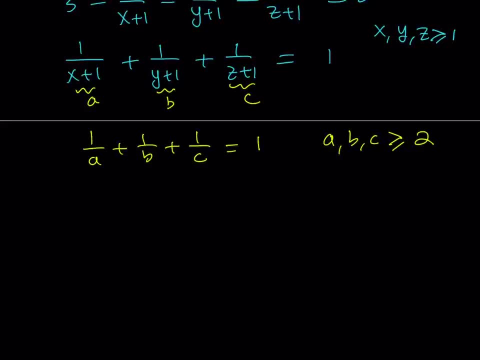 So they're positive integers, but not only that: they can't be 1 either, Okay, So now what we're going to do is we're going to look at this equation, and this is a very special type of equation. 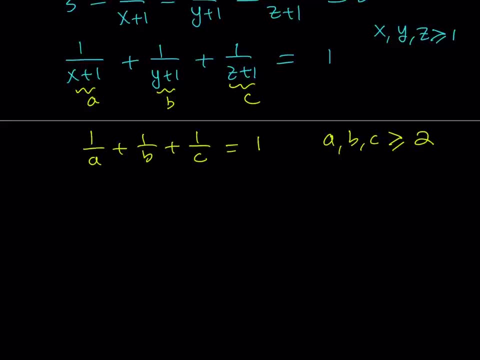 Usually with these types of equations and I think we've done a problem like this when I did a video on Diophantine equations. I'm going to share the link down below. You can look at that. They're very similar, So we're going to use inequalities. 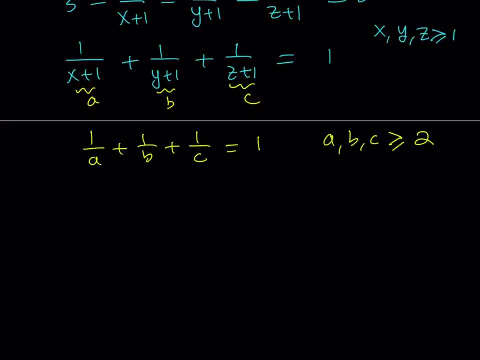 So we're just going to say without loss of generality. of course sometimes people ask: well, what does WLOG mean? It means without loss of generality. So, without loss of generality, I'm just going to assume that. 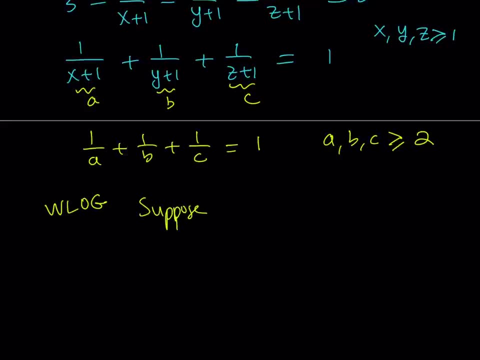 suppose, suppose. I'm going to suppose that a is less than or equal to b and b is less than or equal to c, But this implies that the reciprocals are kind of in the reverse order. So we're going to get: 1 over c is less than or equal to 1 over b, and that is less than or equal to 1 over a. 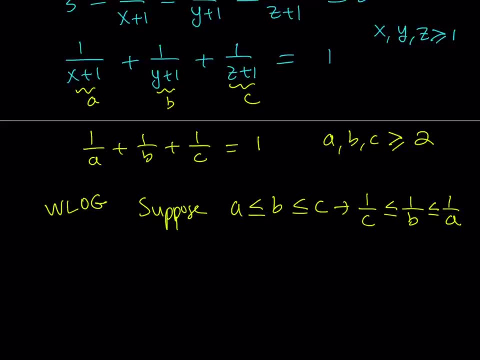 And obviously these are not negative or zero, so it's OK to write them as reciprocals, and the sign is not gonna change. So now we have a really interesting situation here, because we're able to compare the reciprocals. Now what is that supposed to mean? 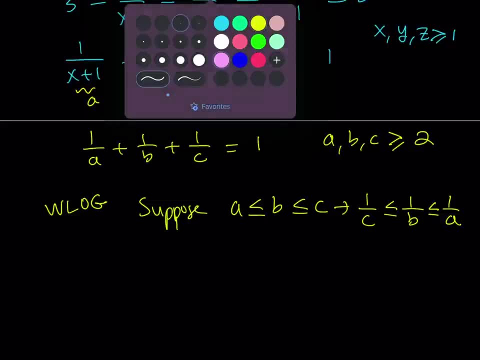 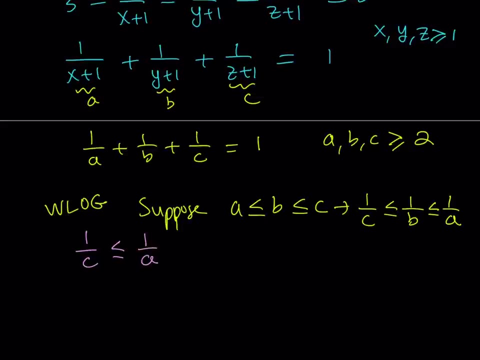 I'm going to be writing a bunch of inequalities to show you what I'm getting at. So the first one is gonna look like this: Obviously, from transitive property, we can say that 1 over c is less than or equal to 1 over a. 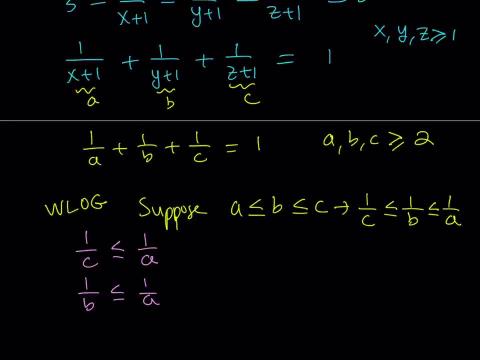 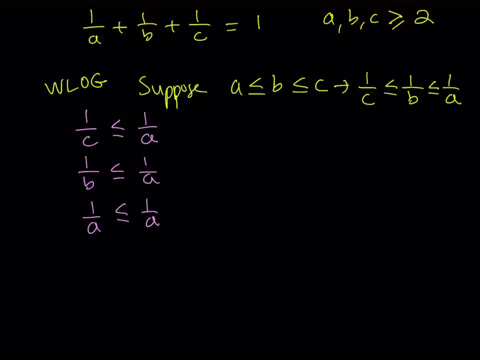 And, of course, 1 over b is also less than equal to 1 over a. Since we have the equality, we can also say that 1 over a is less than or equal to 1 over a. they're not, because they're equal. Okay, Now I'm going to add these inequalities: 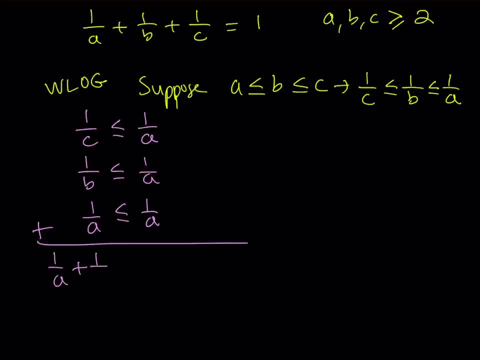 and that's going to give me something super duper helpful. The reason why I do that is because I want to get 1 over a, plus 1 over b, plus 1 over c, And from here I'm getting the a 1 over a. 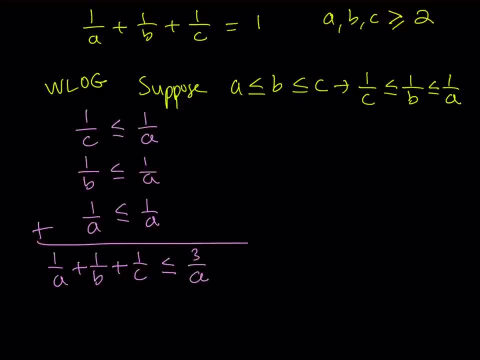 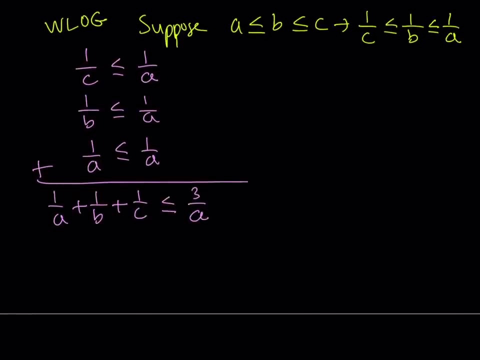 three times. So that's going to become 3 over a. But we know that 1 over a plus 1 over b plus 1 over c is equal to 1.. So I can replace that with 1.. And that gives me 1 is less than or equal to. 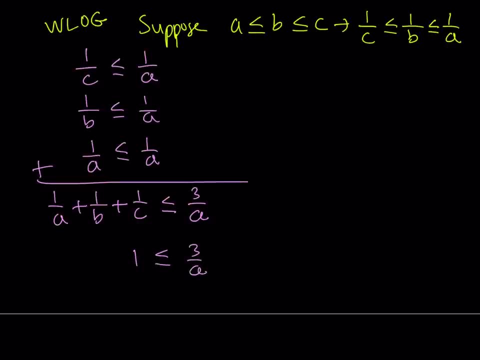 3 over a. If you flip both sides, you're going to be getting a over. 3 is less than or equal to 1, which implies that a is less than or equal to 3.. So this is nice, because we know that a, b, c, all. 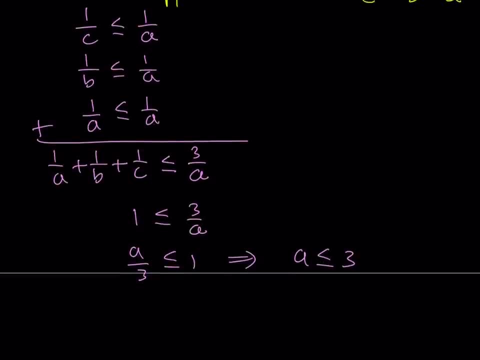 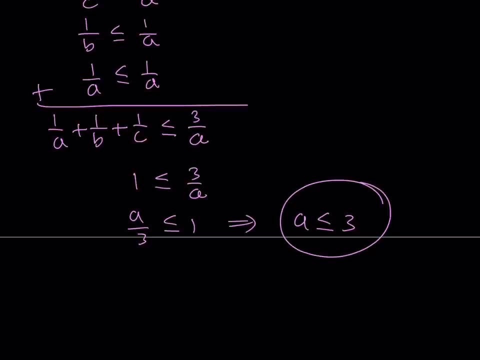 have to be greater than or equal to 2.. And in this case we found that the smallest of these numbers, which is a, in this case, needs to be less than or equal to 3.. So a needs to be basically between 1 and 3 inclusive, which implies that there's only two possible, actually. 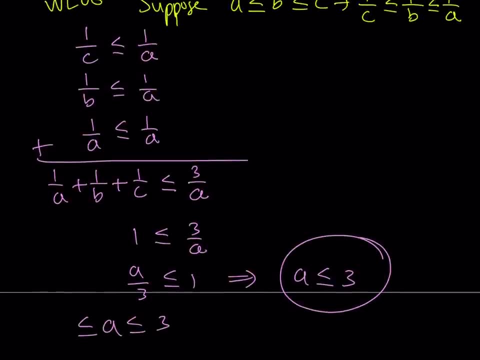 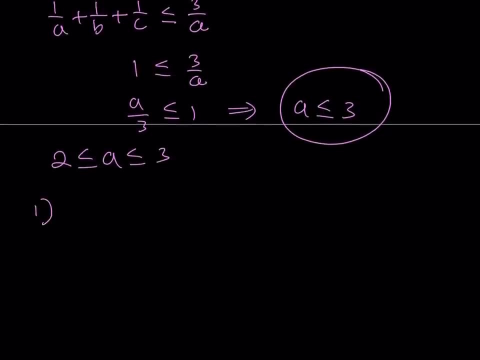 difficulties. It's supposed to be 2, not 1.. So basically, there are only two possible values for a. It can only be 2 or 3.. So let's go ahead and take a look at each case And from here we're going to get. 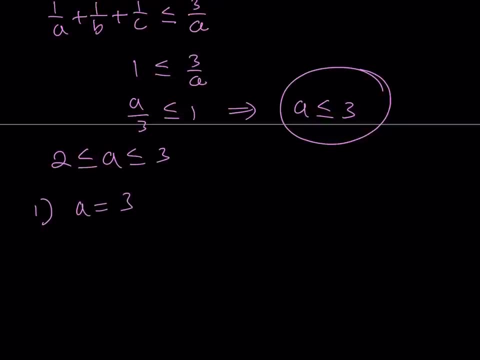 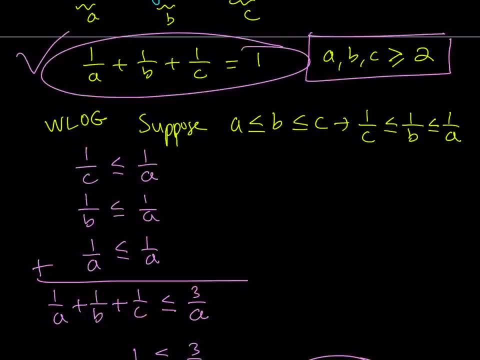 something interesting. Okay, let's go ahead and take a look at a equals 3 first. Now, if a is equal to 3, if you substitute in my original equation- remember well, not the original original, but this one that I got- So the reciprocals: the sum of reciprocals is 1.. So 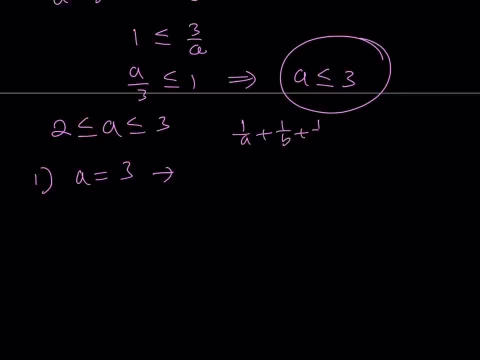 let's go ahead and write that here, So we can kind of look at it as we go. We know that this sum is equal to 1.. Now if a is equal to 3, then I can subtract that from 1 and I get 1 over b plus. 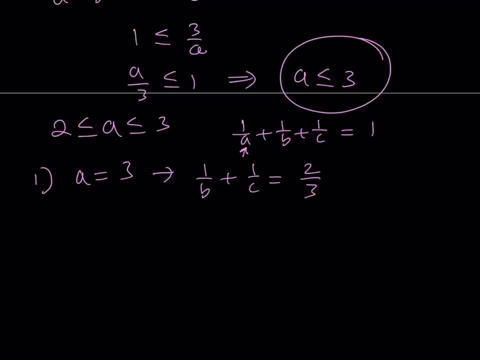 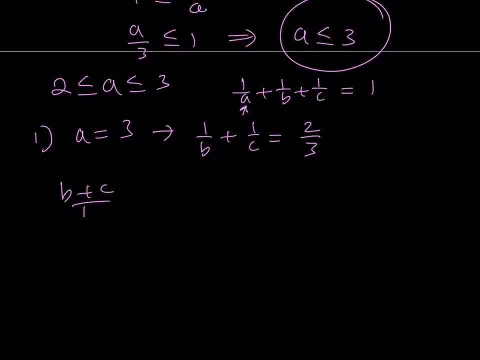 1 over c is equal to 1 minus 1 third, which is 2 thirds. Now this equation can be solved. But let me go ahead and get into a little bit of details. here We can make a common denominator because 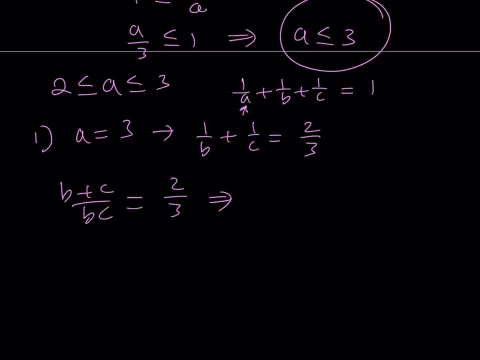 we're going to be using something real cool And that is actually called Simon. Let's go ahead and do that. So we're going to cross multiply here. I'm going to be getting: 2bc is equal to 3b plus 3c, So I kind of got the 2b here, right, 2bc. See, I got 2bc, So let's go ahead and put. 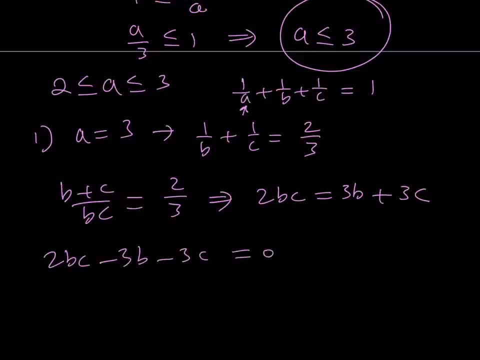 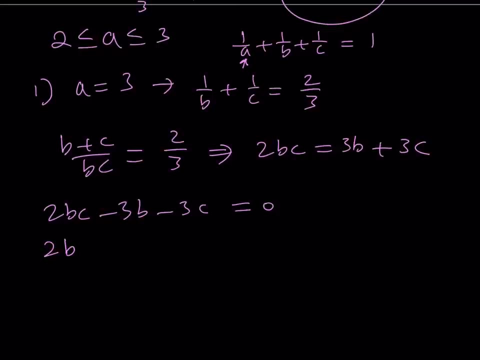 everything on the same side and set it equal to zero, Nice. So in order to solve this equation, I would like to take out a 2b. You might be asking: why aren't you taking b? You could do that too, but it's better to take out 2b so that I can start with c here inside the parentheses. 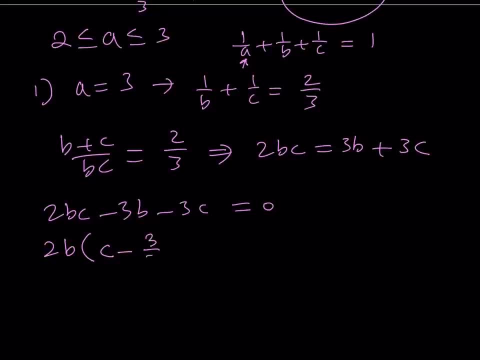 minus. So I got to adjust a little bit here. I do need three halves Minus three. Now I got to get the same thing here. I need to get the same thing so that Simon works. So I need to subtract three halves, But notice that I'm adding negative three times negative three halves to both. 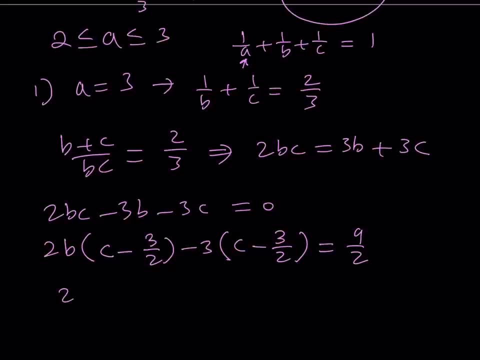 sides, which is nine halves. So this gives me 2b or not. 2b, Yay. 2b minus three times c minus three halves is equal to nine halves. If you multiply both sides by two, you get 2b minus three. 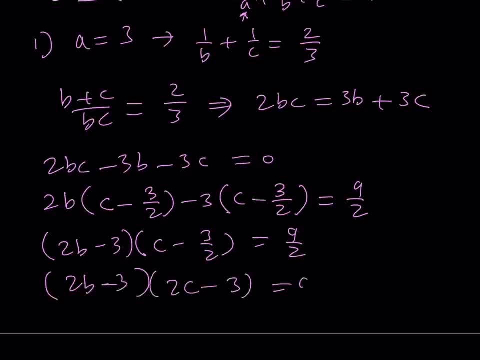 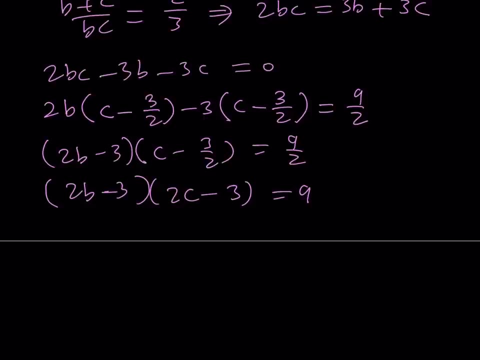 multiplied by 2c minus three equals nine. Now we're going to look at factors of nine. Of course it's going to be positive, because if one of these is equal to negative nine, for example, you're going to get a negative answer. So it's not going to work. So we can have the following: 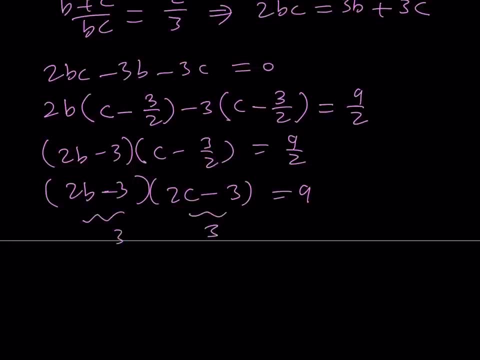 situations, Both of them can be three. From here we get b equals three and c equals three, Or one of them can be nine, The other can be one. In this case, b is going to be six and c is going to be. 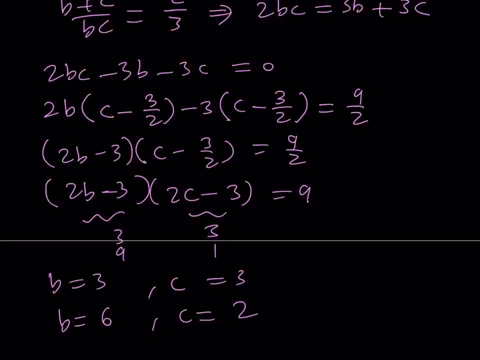 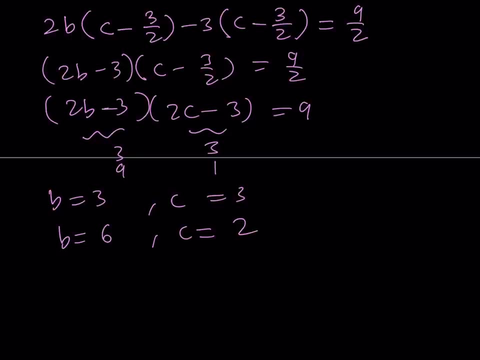 two. Now do I need to consider the switches Later on? I'm just going to go ahead and consider all of that, So we don't need to worry about it right now that b and c are interchangeable. So we got these values, But remember our a value was three, So we know that. 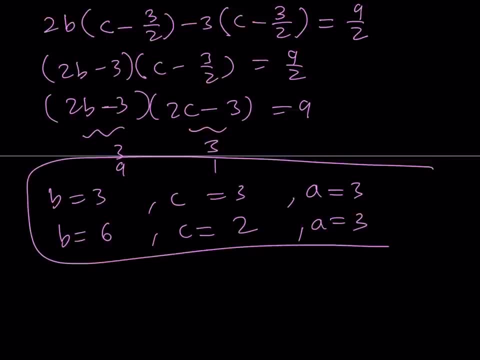 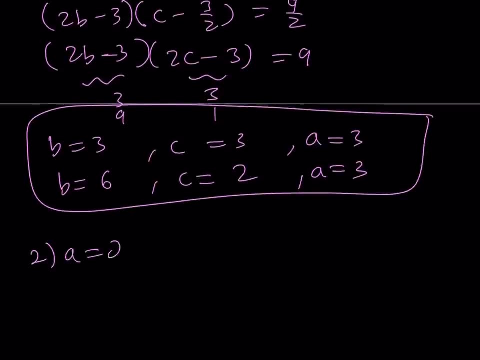 a is three here in both of these cases. So that's one of the things that I find first All right. Let me go ahead and take a look at the second case scenario, which is when a is equal to two. Now, if a is equal to two, then in my original problem, remember, it was one over a plus one. 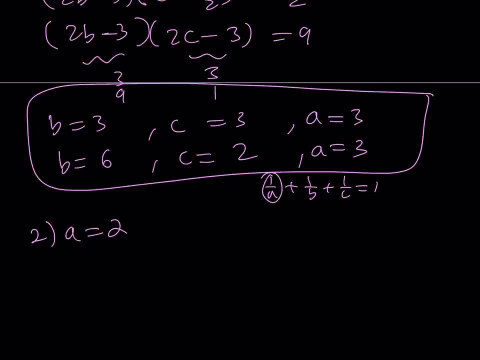 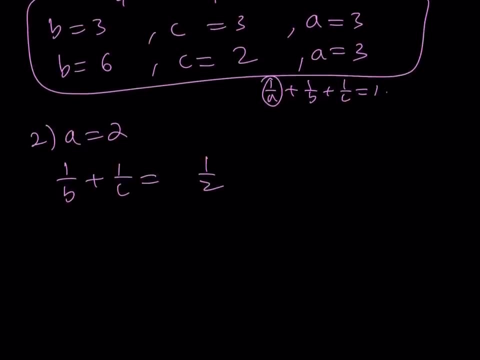 over b plus one over c equals one. If you subtract one half from one, you get one over b plus one one half. So this equation again is easily solvable. But let's go ahead and look at the cases. Let's go ahead and use Simon again one more time: b plus c over b c is equal to one half. 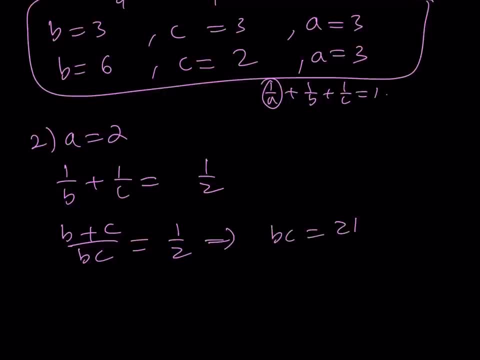 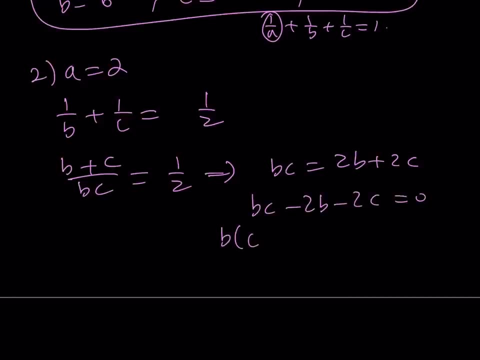 If you do the cross multiplications you get b, c is equal to two b plus two c. And then from here, b, c minus two, b minus two c is equal to zero. And if you use Simon, we're going to get something. 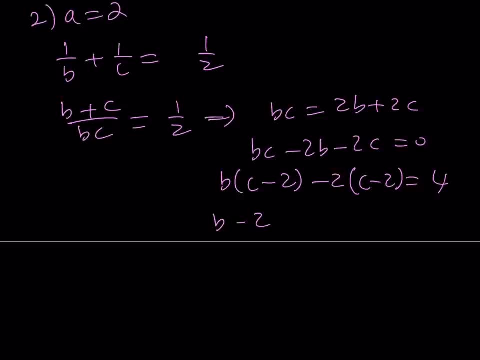 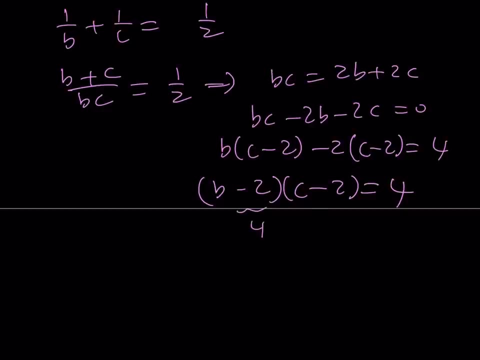 like this: I'm adding four to both sides, And this gives me b minus two times c minus two is equal to four. Great, And from here obviously we have two cases. Either we can have four and one, which means b is equal to six and c is equal to three, Or we can have the two, two, And that means 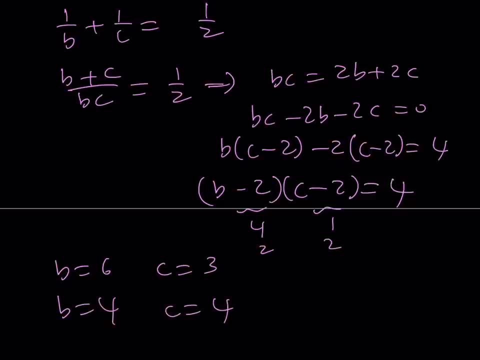 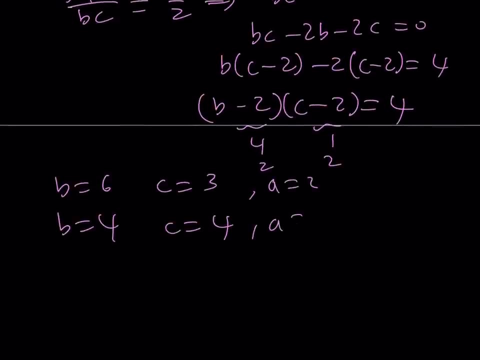 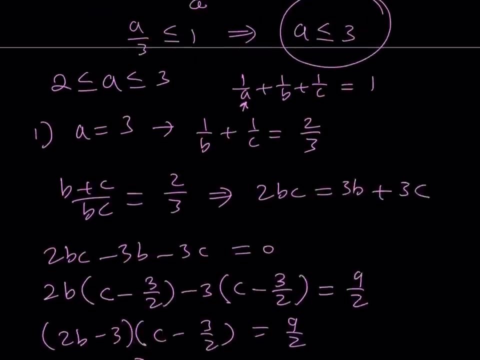 b is equal to four and c is equal to four, So they're going to be equal in this case. But of course we already have the assumption that a is equal to two. So those are going to be my second batch. Now. that's pretty much all the solutions, because we know that a needs to be, if you remember. 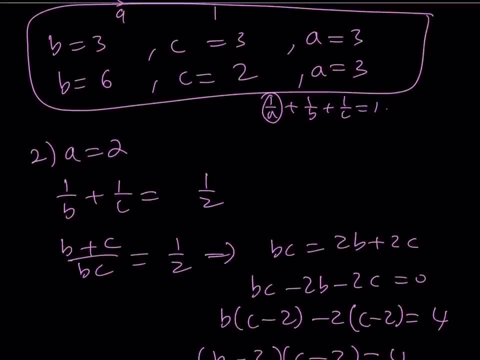 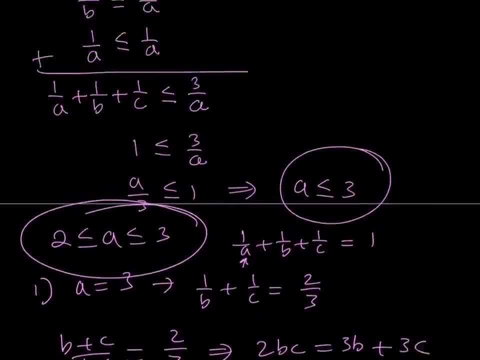 a needs to be one of these values. So that's pretty much it. But here's the thing. I got these values. But let me go ahead and write the x, y, z values, because we use substitution to get to a, b, c. And what was that? we said that, okay, let x plus one equals a. So that means x is equal to a. 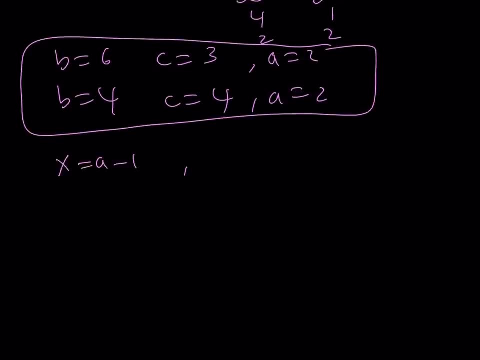 minus one. obviously right. y is equal to b minus one and z is equal to c minus one. So what we're going to do is we're going to be subtracting one from each of these values and then get the answer. so let's go ahead and do that, starting with these ones. So if- and I can just write it as a set, so 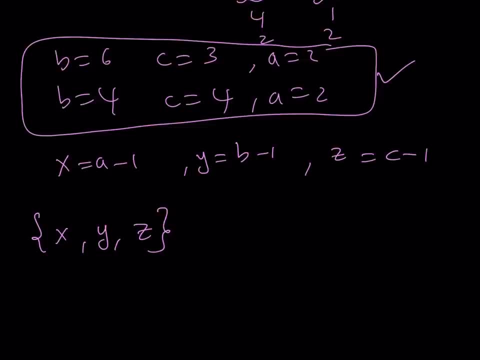 that I'm switching. I'm actually considering all the switches, because x y z are all basically interchangeable. So from here I get that x, y, z as a set can be- since I'm going to be subtracting one from each of these values. it can be one, two and five as a set, or it can be one, three and. 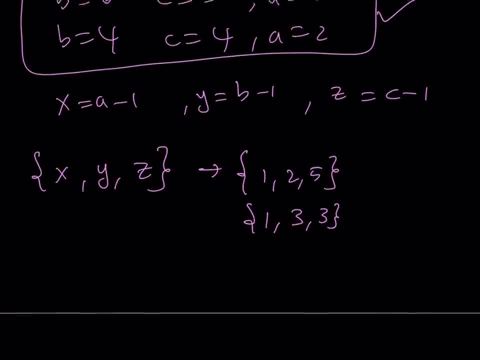 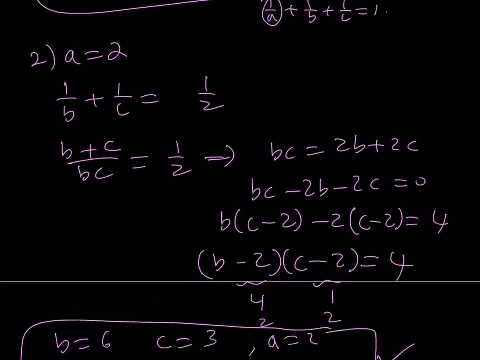 three. of course, they can just switch around. Or I have the other situation where I got three, three. let's go ahead and write that down here. I got the three, three, three, and the other one was three, two, six, three, two and six. Those are ABC values. by the way, what I'm going to do, 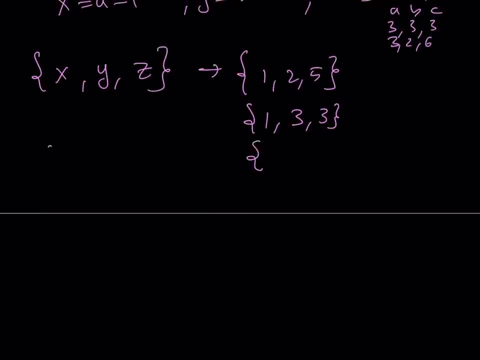 is, I'm going to subtract one from each of them to get the x, y, z values, And that's going to give me two, two and two, right. And then the other one is going to give me two, one and five, But of 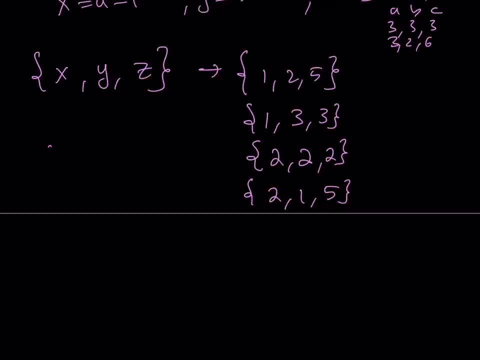 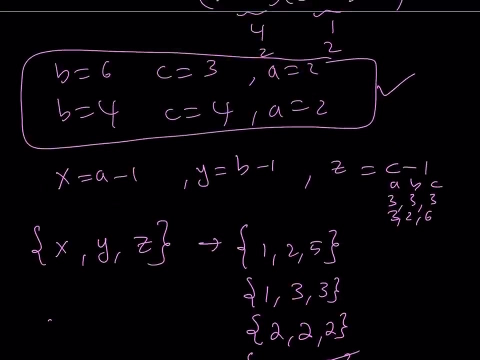 course, when you consider the one two five and the two one five, that's basically going to give you, so it would not matter. So we only need to consider these three situations. All right, And this brings us to the end of this video. Thank you for watching. I hope you enjoyed it. 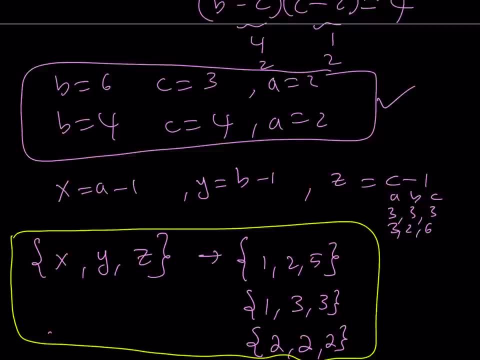 Please let me know what you think. Don't forget to comment, like and subscribe. I'll see you tomorrow with another video. Until then, be safe, take care and bye. bye.